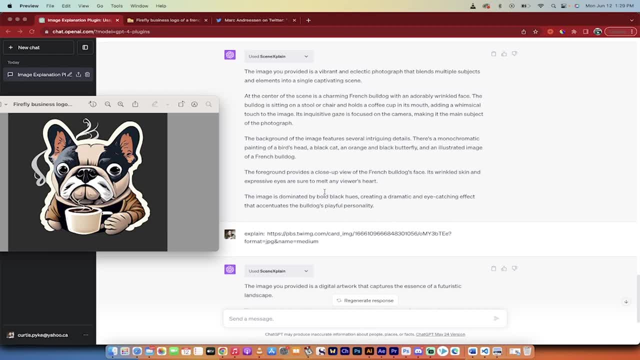 Hello everybody, Welcome back to another AI video. In this one I want to talk to you about SceneXplain. This is a ChatGPT4 or a ChatGPT Plus plugin that you can now download And it's very similar to MidJourney and other where you can describe with text. You can reverse engineer out. 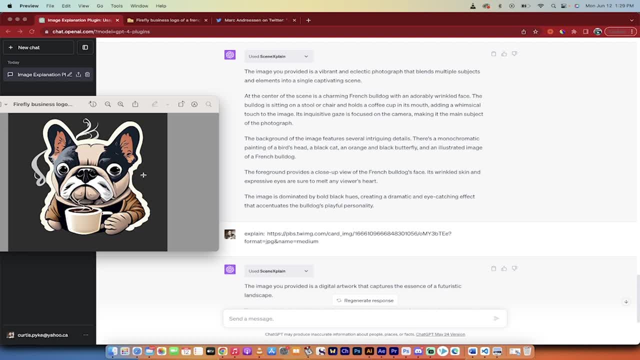 the description from an image. Look at this. I've got a bulldog here with a cup of coffee and, like these butterfly type look in his ears. And I asked ChatGPT, using the SceneXplain plugin, to explain to me what this image looks like. And here's what I came up with. It says: the image you. 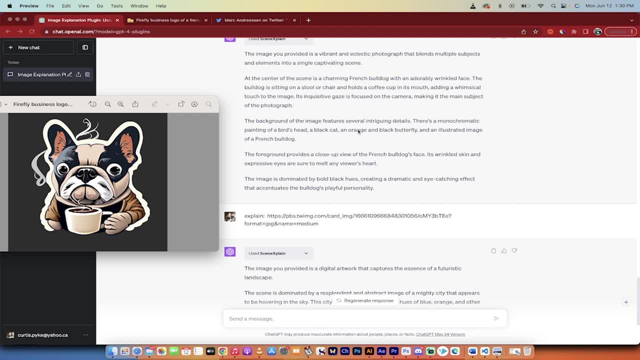 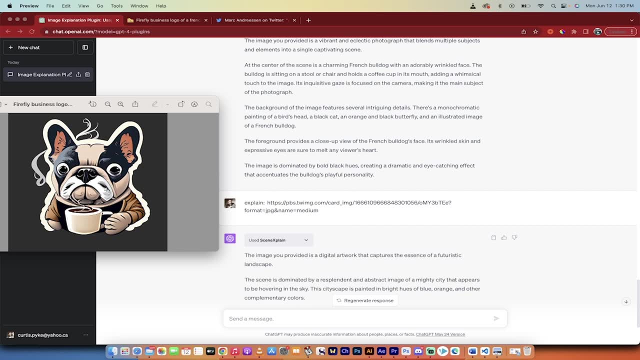 provided is a vibrant and eclectic photograph that blends multiple subjects and elements into a single captivating scene. At the center of the scene is a charming French bulldog with an adorably wrinkled face. Check, That's correct. The bulldog is sitting on a stool. He is not or. 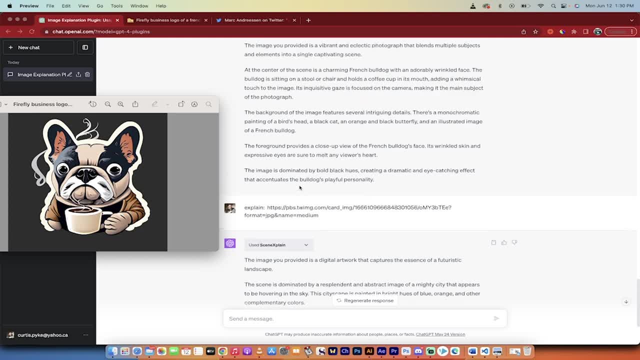 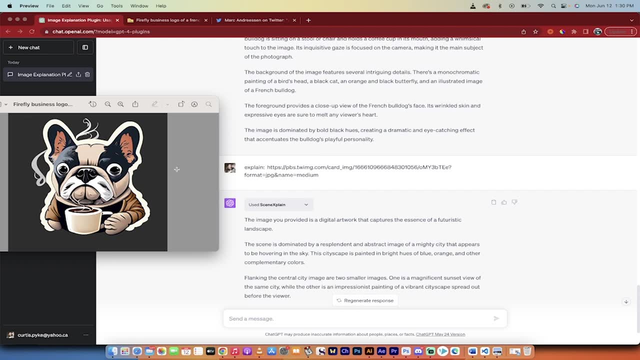 she is not, But in the original image, before I cropped it, there was a stool And it holds a cup of coffee in its mouth, which is pretty close as well. And there you go. So I basically reverse engineered what the text is. or, if you're doing prompt generation or AI art. 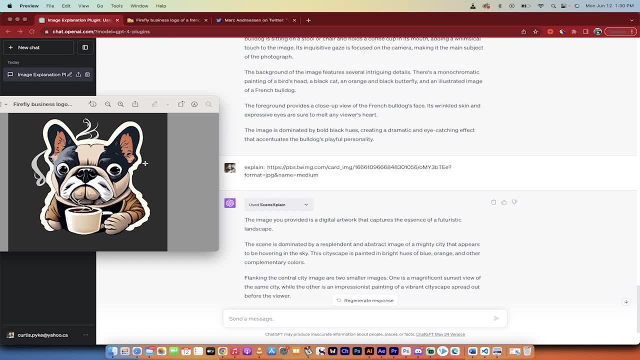 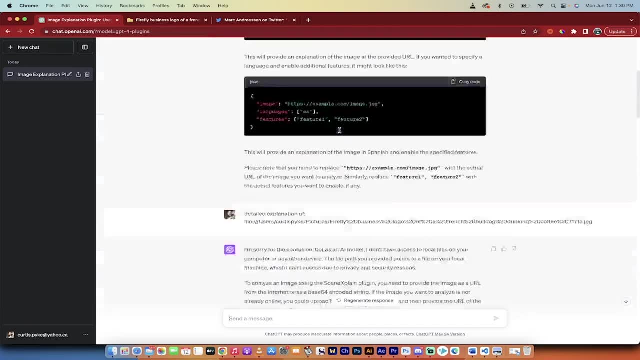 generation what the prompt is that you can use to create something like this. This was done in Adobe Firefly, for example, And, yeah, let me show you how to use it. So the first step here is: you need to go. Let's just create a new chat and start from scratch. First step: make sure you're selected. 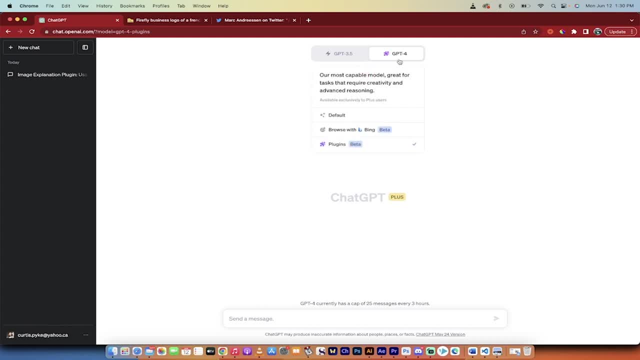 here. Now go down to the plug ins, click on the plug ins and make sure that there's a check mark beside plug ins. When you do that, you're going to see this little square, this little rectangle here, And you can now click on that and it'll tell you what plug ins are installed. I've got scene. 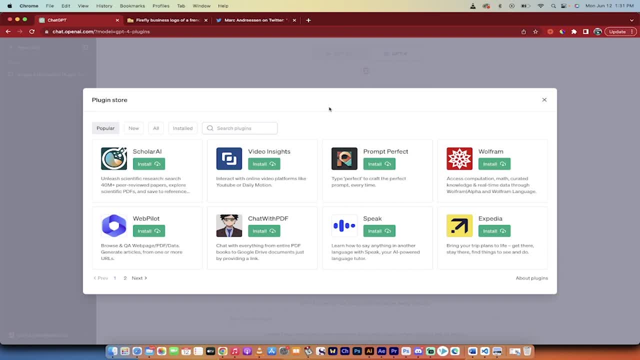 explain: installed. There's a check mark beside it. You can click on the plug in store and you can always click on installed. And if it is not installed, you just want to basically search for it right here, Just type in scene and presto, You can install it. Click on the install button, That's. 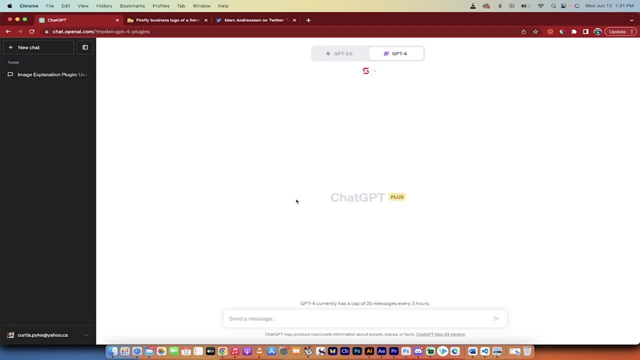 OK, That out of the way. Here comes a bit of the. there's two things you can do with this plug in. The first one is you can basically go ahead and find an image on the Internet and have it describe that. That is the easiest way And that's the way I recommend in most cases, unless you have your own. 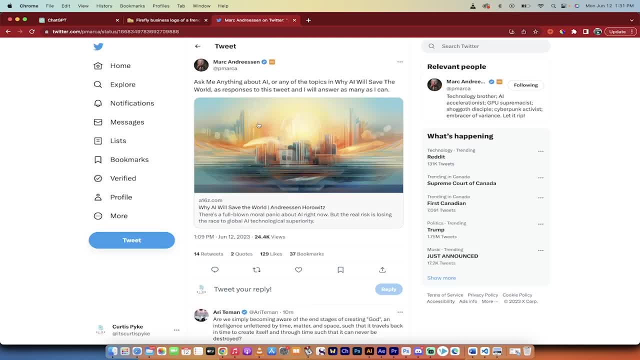 images that you want to show, And I'll show you how to do that as well. So here we go. I just went on to Twitter and one of the images that popped up was this one here: Mark Andreessen's got an image here on Twitter. What I'm going to do is I'm going to right click on this image and then I'm going to 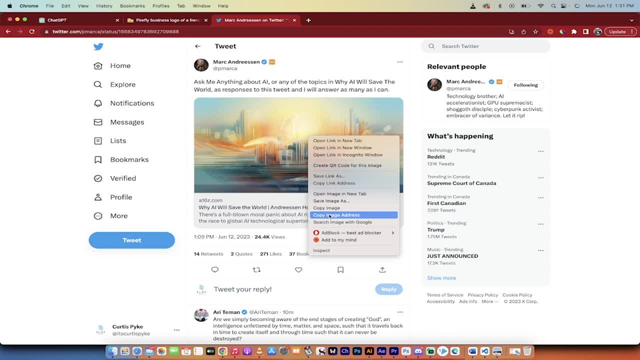 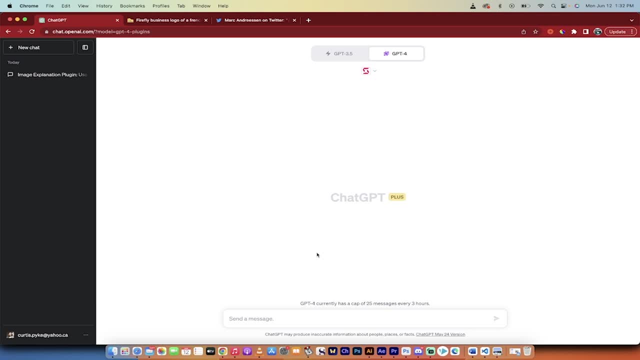 copy image address. It's very important that you copy the image address, not save it or any of those other things. Copy image address. Go back into chat GPT again making sure scene explain is available and use and being used and go explain this image. Semicolon command V: copy paste that. 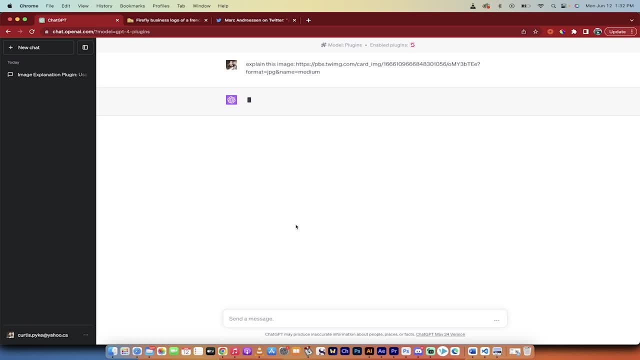 in and scene explain, is going to go ahead and do its best job to try and explain that image off the Internet. So that is the first one. The second one: What I need for that is, I want to show you the second method, And there are no doubt many ways to do. 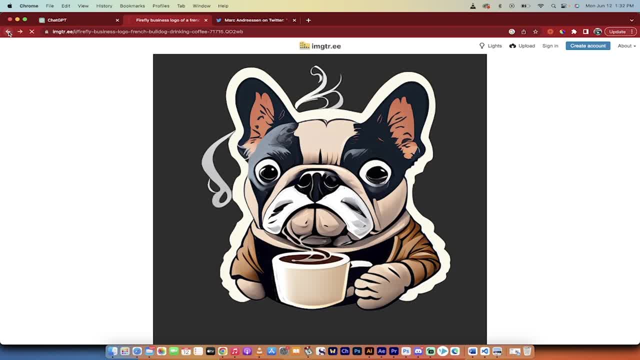 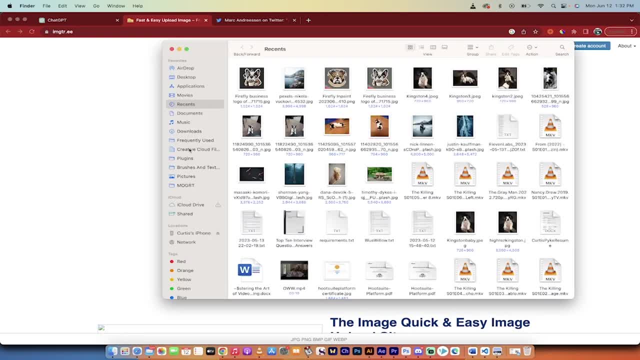 this, But the way I found that worked best was using this free website called Image Tree. Image Tree allows you to drop, and basically just drag and drop one of your own images. So in this case, I'm going to do the same images last time. I'm going to grab my pictures and then I'm going to 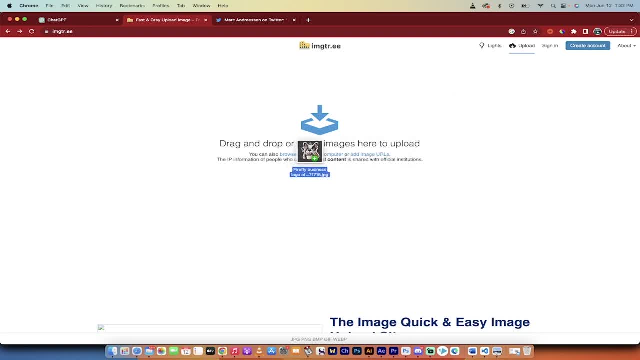 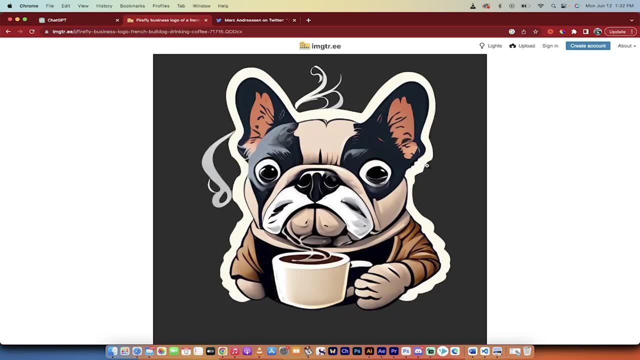 grab this JPG of this little bulldoggy doing bulldog things: drinking coffee. drag and drop it right there. When it's done, I'm going to click on Upload. It's going to upload it And then when I look at it, you're going to see here that I can go ahead. 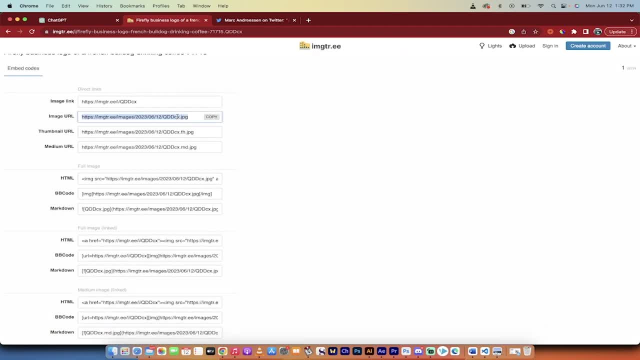 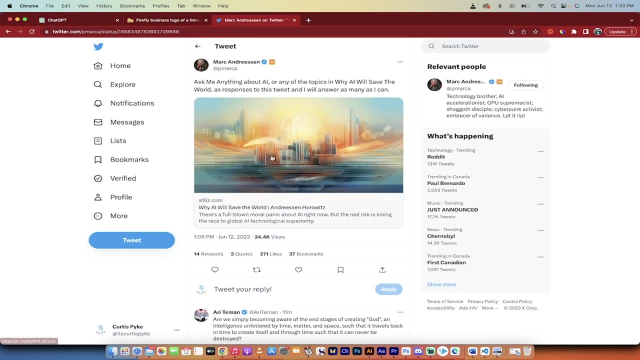 and do a few things, But when I go, when I scroll down, you're going to see here that it gives me an image URL. So just keep that in the back of your head. Let's go back to the original. So this one and this is the original image. Take a look at it here. This is what scene explain has told. 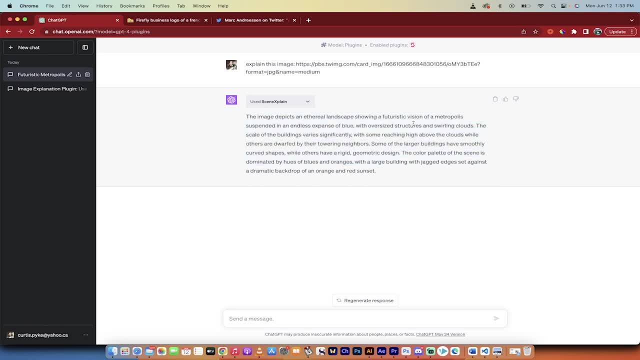 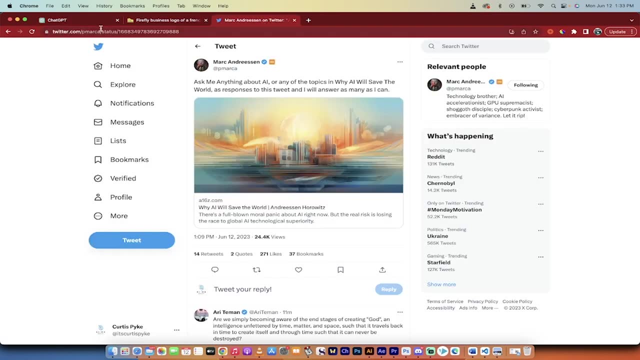 us about the image. It depicts: an ethereal landscape showing a futuristic vision of a metropolis suspended in an endless expanse of blue with oversized structures. You know what It hit the nail on the head here pretty good. So that's the first method, The